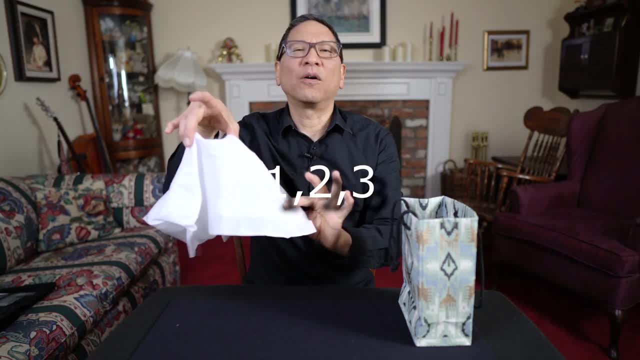 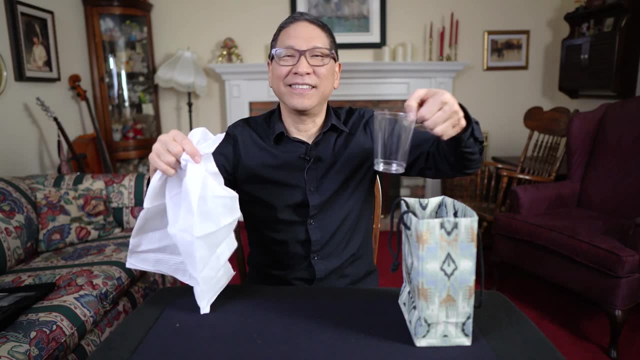 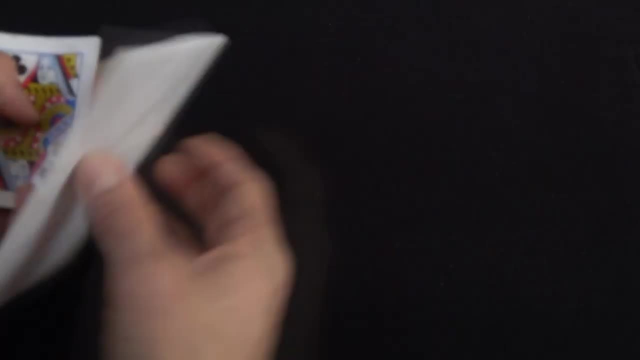 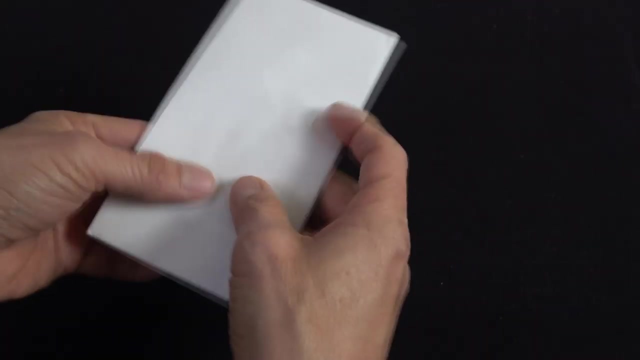 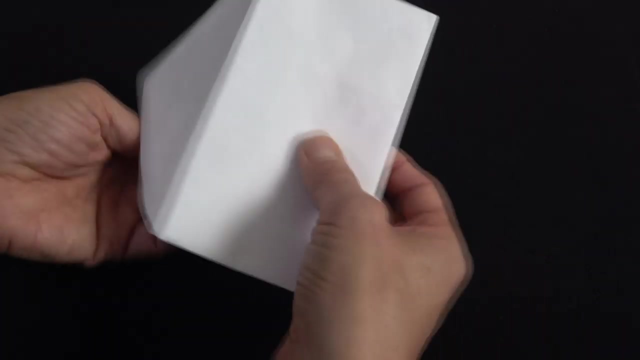 I'm just going to go snap my finger and go. one, two, three And you'll find the cup right here inside the bag. Two queens, a couple other cards. Goes into an envelope. Magic Move a queen. Move a second queen. 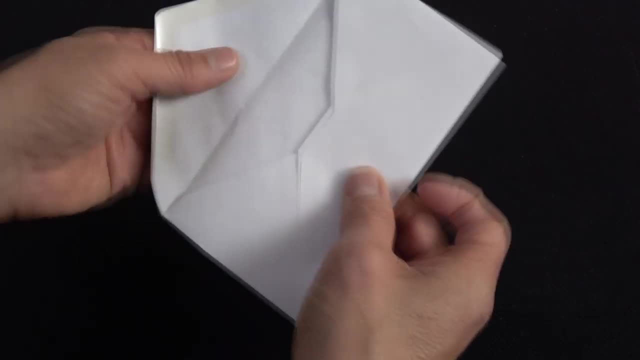 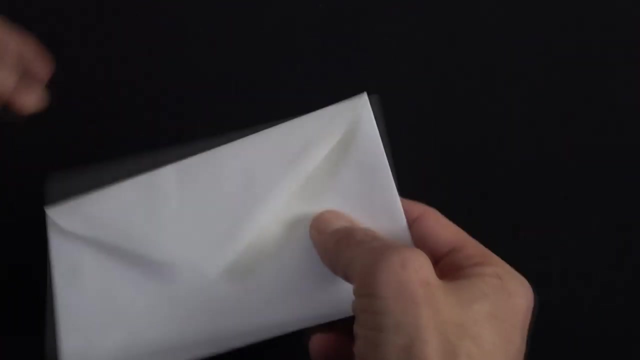 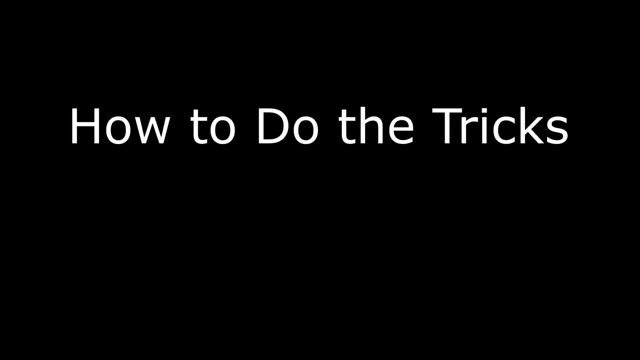 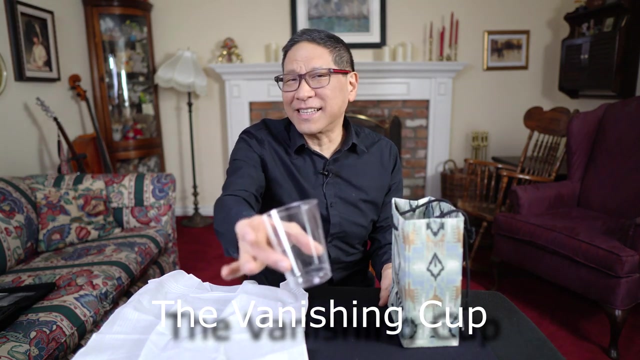 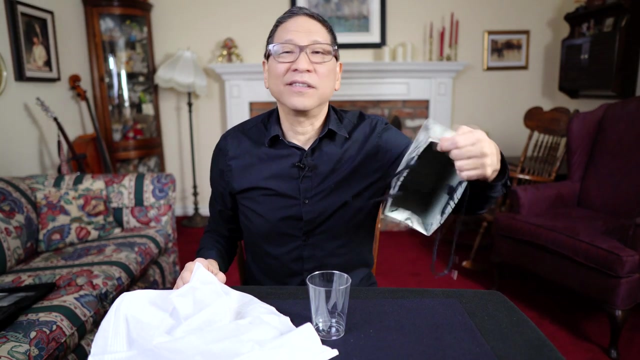 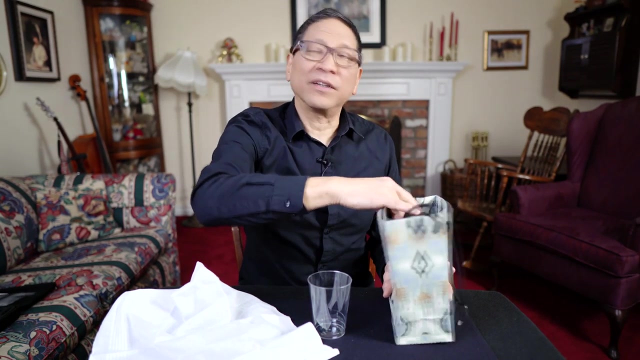 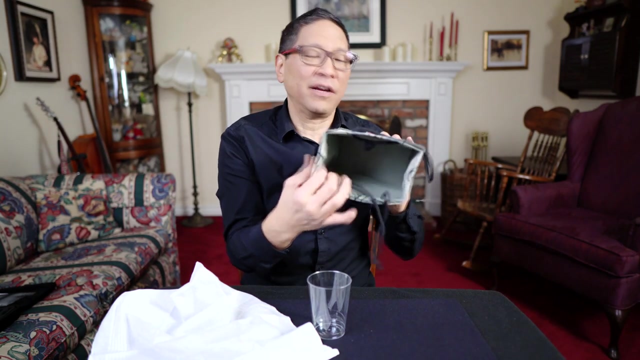 What's left in the envelope? Absolutely nothing. There we go. Here's how to perform the trick. What you're going to need is: you have here. the trick is you're gonna give away the secret, but all you need is an ordinary. I just haven't used gift bag. you can use a hat. that's actually the. 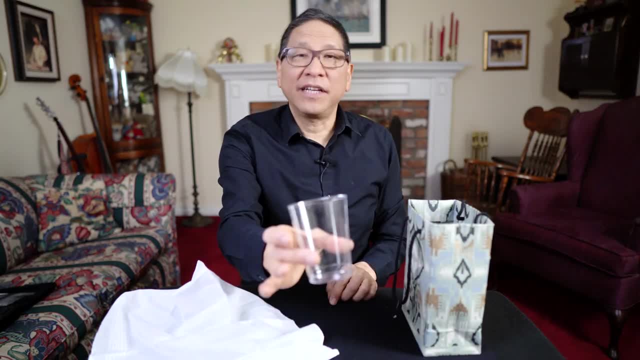 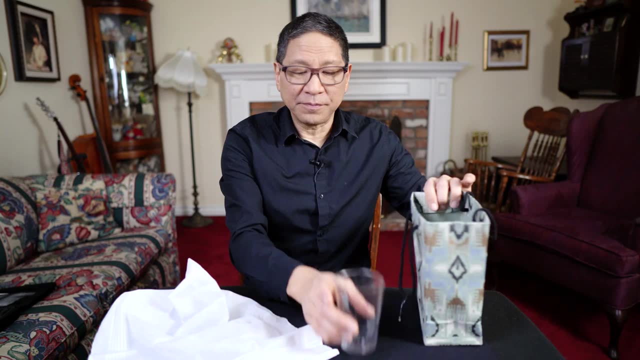 classic way to perform the trick. gonna need a cup- actually any cup, it doesn't have to be clear. I just happen to use a clear plastic cup here and you have a napkin or handkerchief, but this is gimmicked ahead of time. what I've done 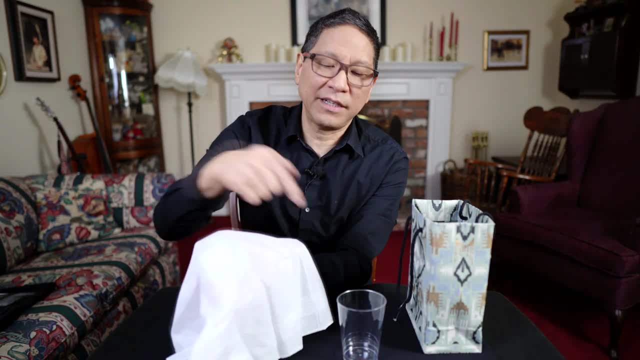 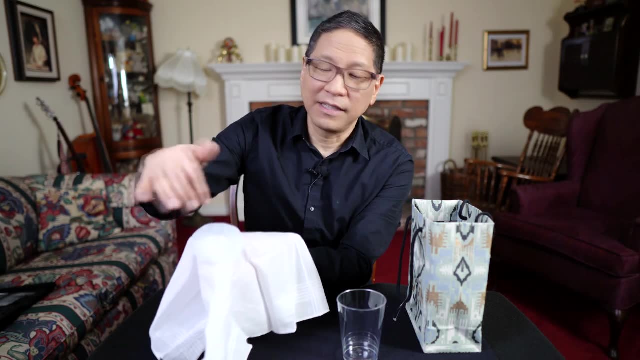 was. I don't know if this might be a little hard to see, but what I did was I took outlined on a piece of. I happen to use part of a drink lid. that's plastic, but you can also use a piece of cardboard, it really doesn't matter you. 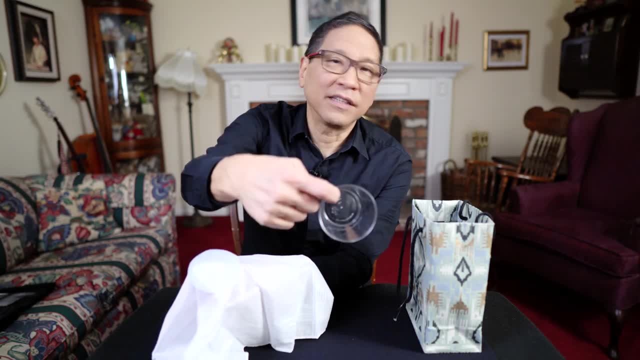 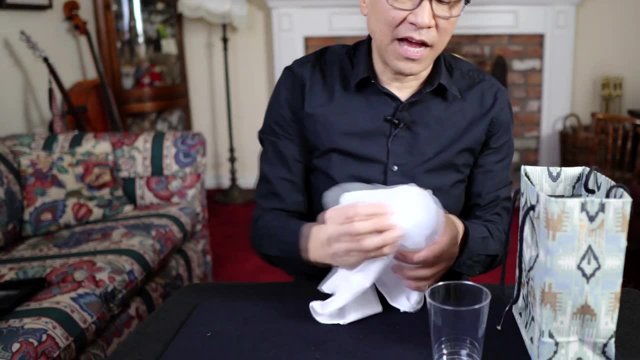 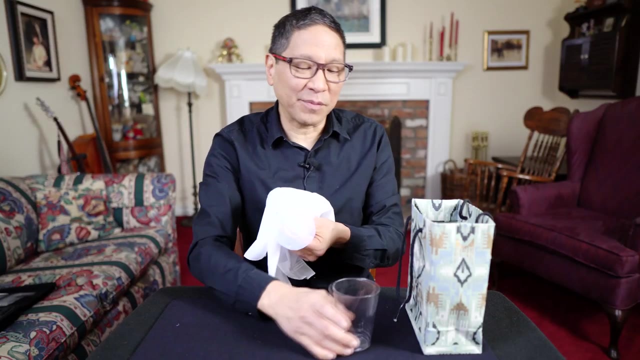 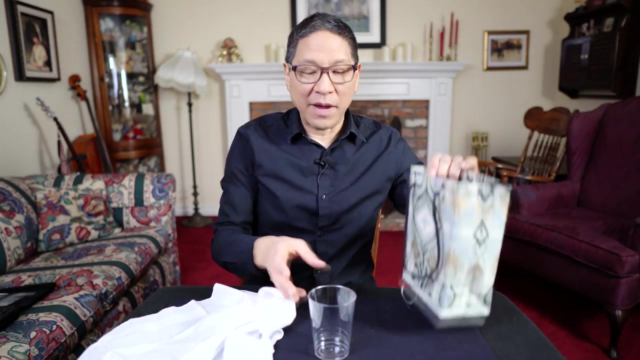 outline on the cardboard the diameter of the cup mouth. so what I've done is this piece of plastic is the same size as the mouth of the cup here and you're ready to perform the trick. just have your handkerchief lying down on the table, you show your bag, show your glass and then you say you're going to. 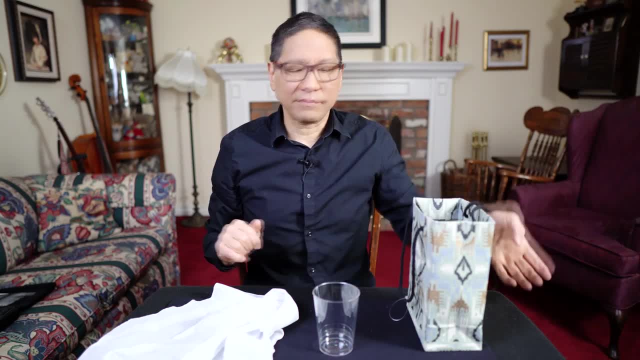 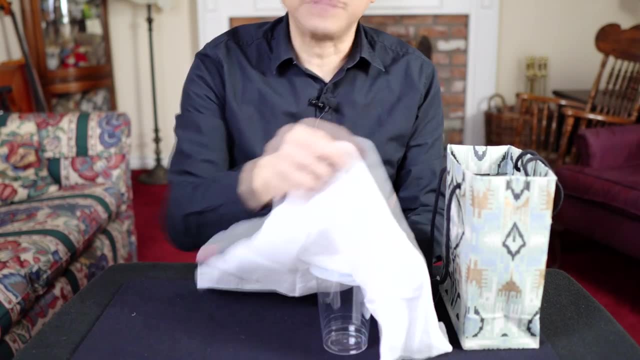 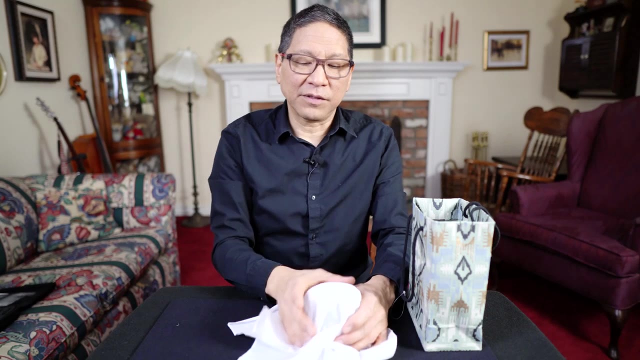 try and make the cup magically go into the bag. take your handkerchief, place it over the cup and what you want to do is make sure that the plastic disc, or cardboard disc, is right on top of the mouth of the glass. now, under cover of the handkerchief, you lift everything: the cup and your disc. 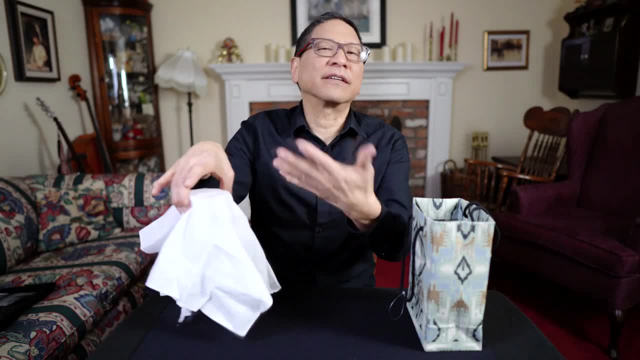 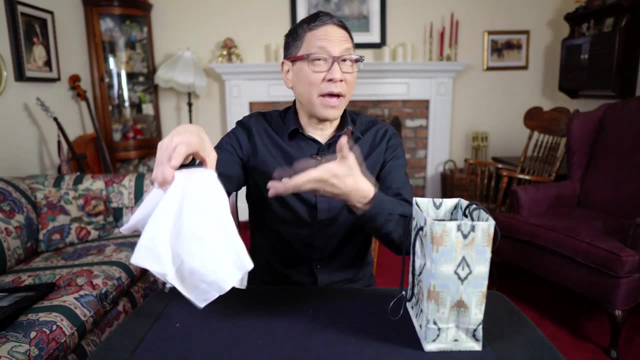 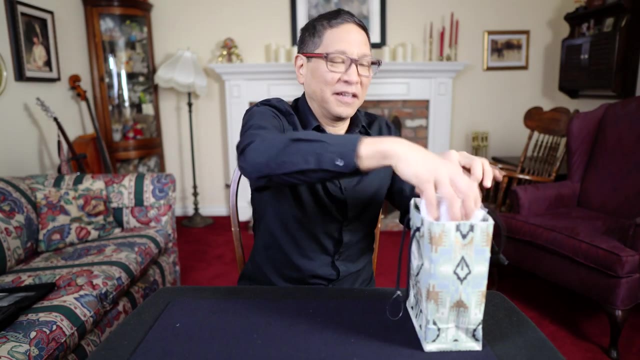 together. you want the spectators to kind of get used to the idea of a cup being under the handkerchief. now you say I'm going to magically place, cause the cup to go into the bag, and then you just go ahead, put it in the bag and you go: oh, that's not what you had in mind. is you really wanted a? 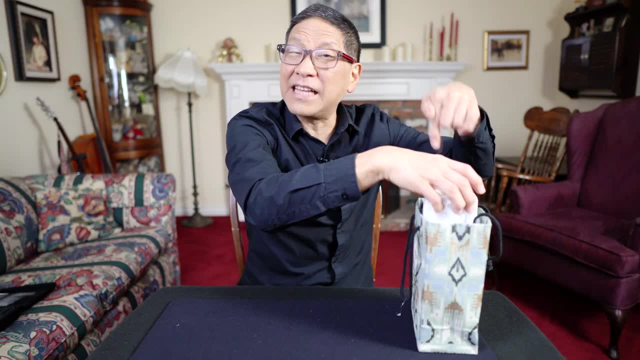 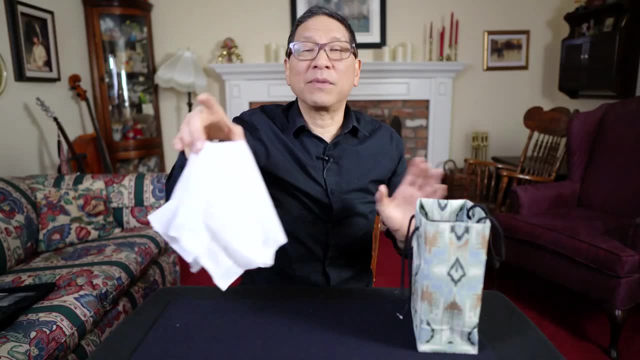 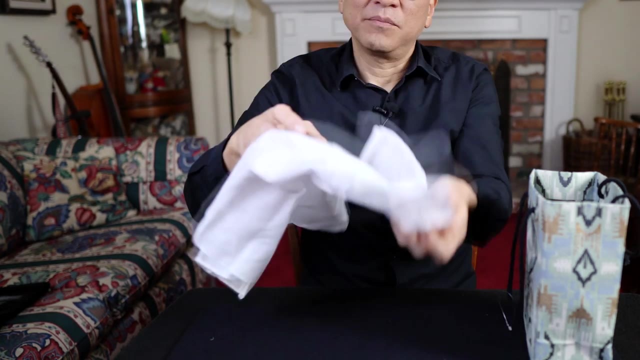 magical way. now, at this point I've left the glass in the bag and now I'm just gripping that plastic disc- or in your case it might be cardboard, but so you can see the disc here. but you can see that the disc actually looks a lot like the. 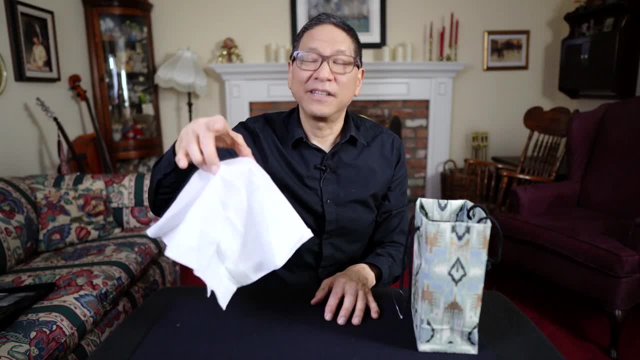 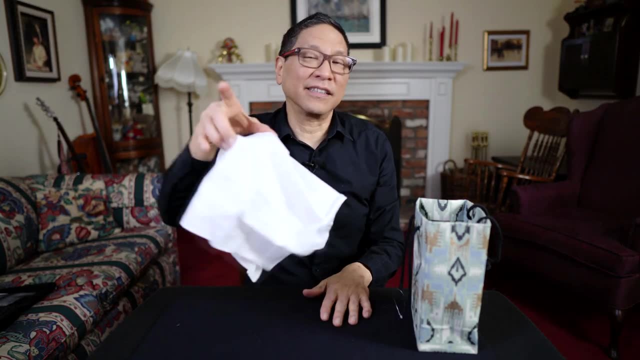 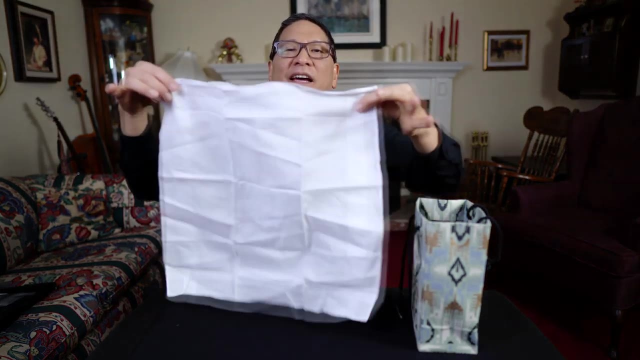 like there's a glass underneath the handkerchief and that's the secret. but of course the glass is already in here. I left it there and I just have this disc here acting like it's the glass, and then when I want to make the Vanish, I snap my finger, I just grab the napkin and it seems to vanish and then I can show. 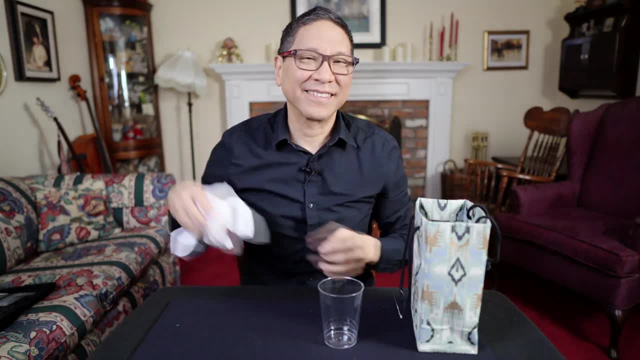 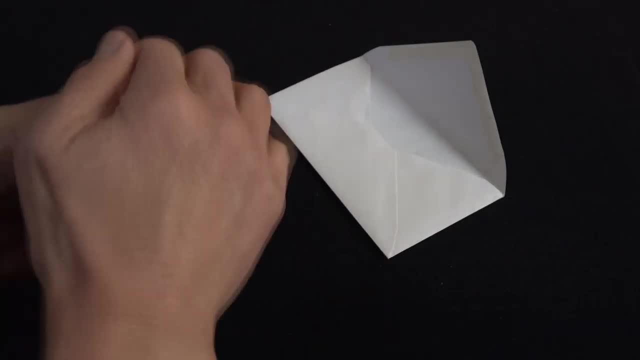 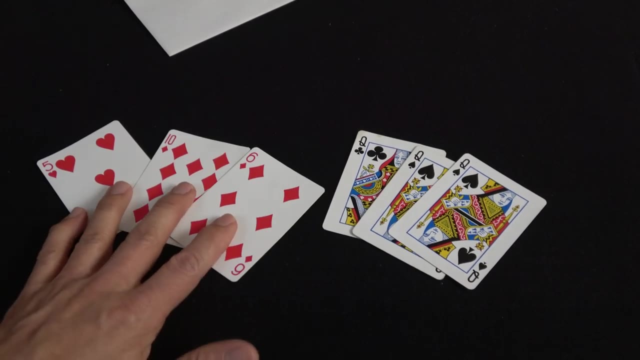 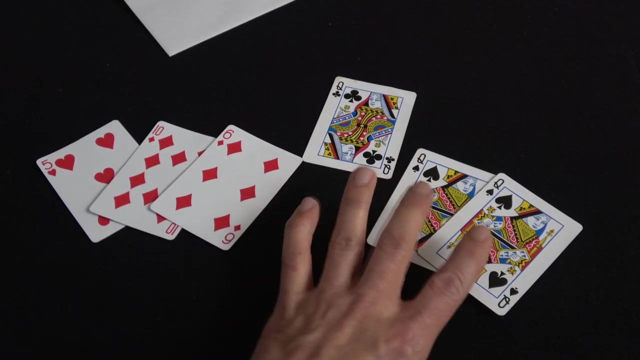 the glass inside of the bag. for this trick, you're going to need an envelope- three in different cards- and we're using Queens here, but the key point is that you can use any cards that you wish, but two of them have to match, so in this case, I have two queen of spades. 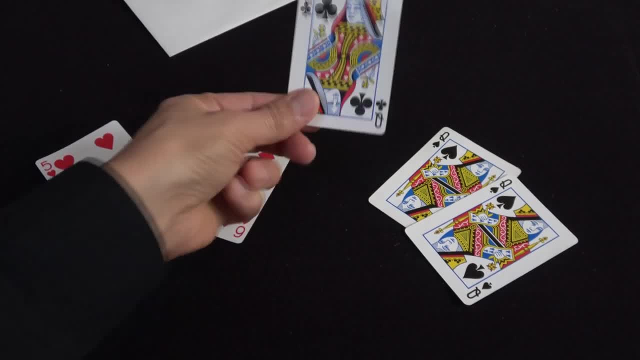 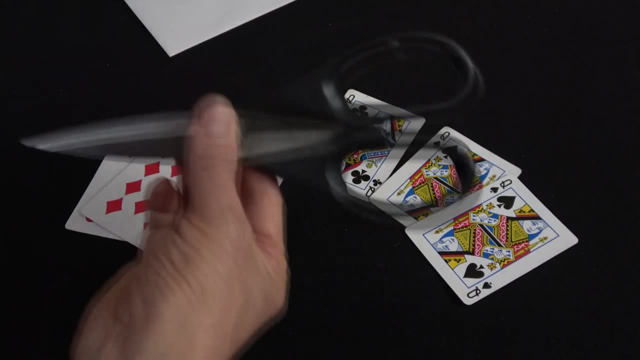 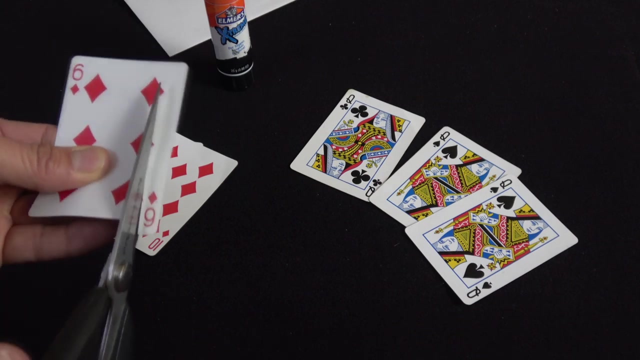 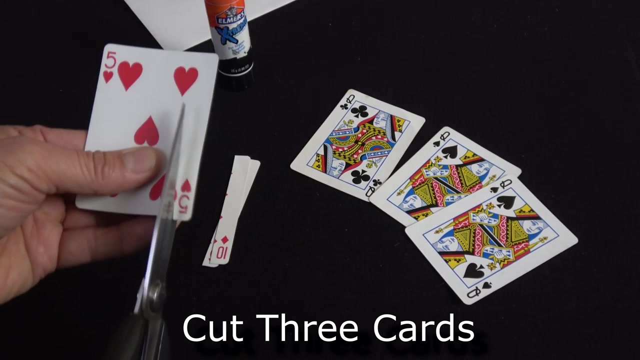 a queen of clubs- I like these to be Queens or Jacks or Kings, because I think it just, uh, plays a little better- and three in different cards, and you'll need scissors and you'll need some glue taking. You're going to cut right along here a thin strip. 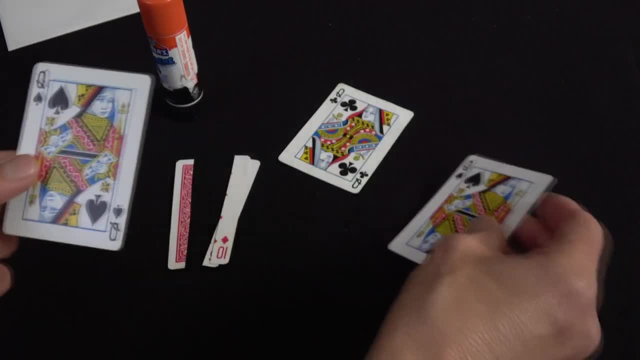 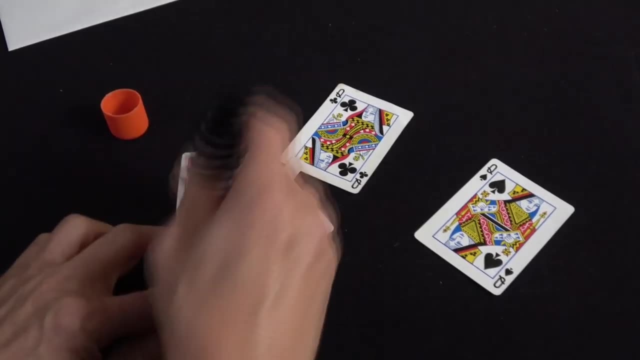 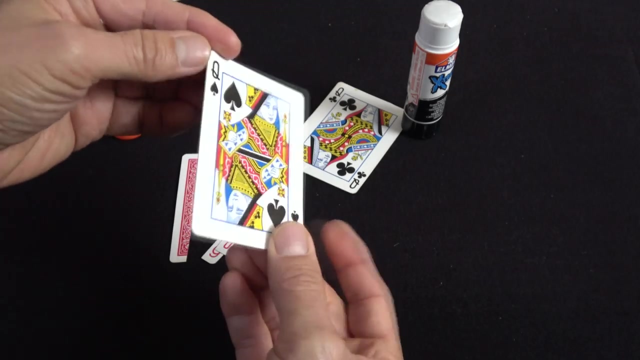 Now take your matching cards. I happen to be using the Queen of Spades here, and what you're going to do is glue the Queen of Spades back to back, So you now have a gimmick card with a Queen of Spades on both sides. 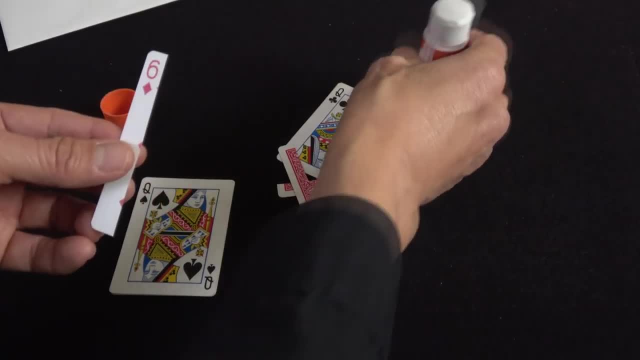 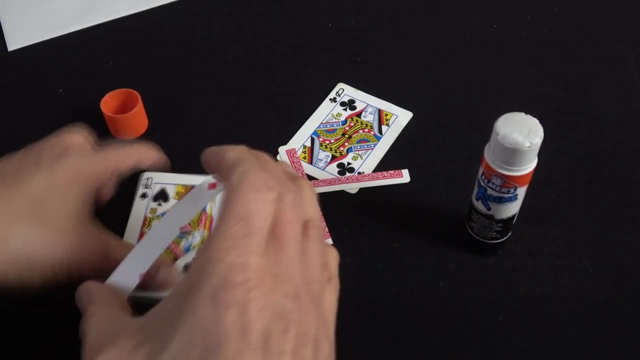 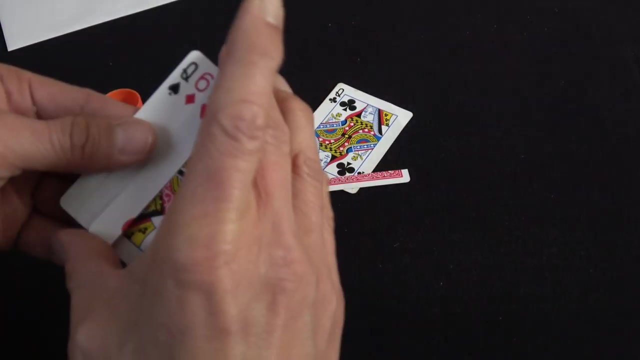 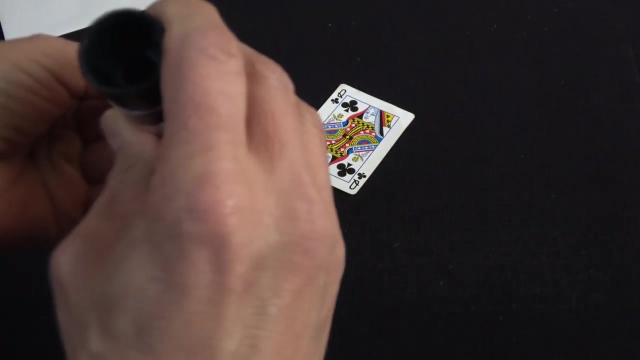 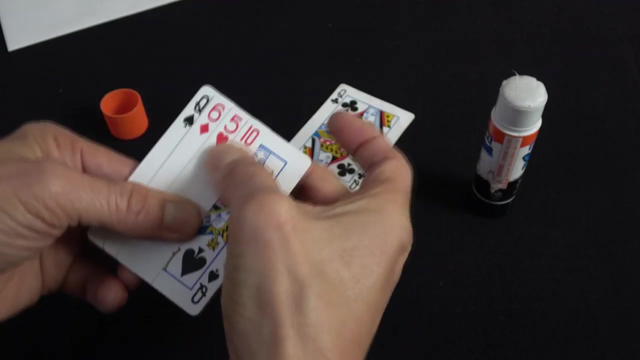 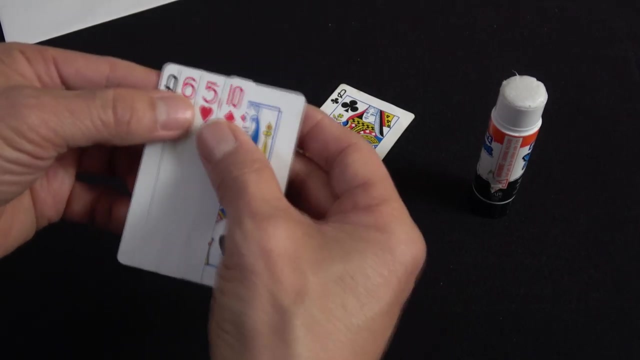 Now, on one side of this gimmick card. you're now going to glue these strips from the other playing cards in a peculiar way: Glue one there, Next one there, Last one, Let it dry and you have a gimmick card that looks like this: 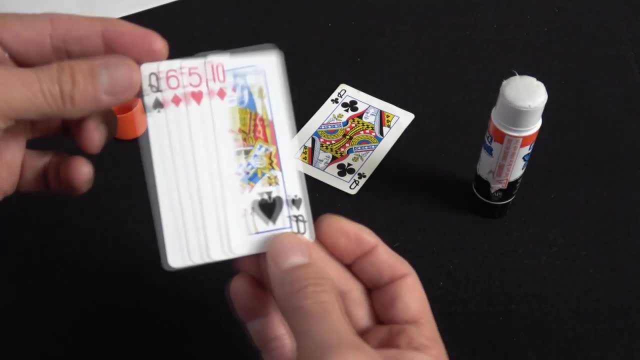 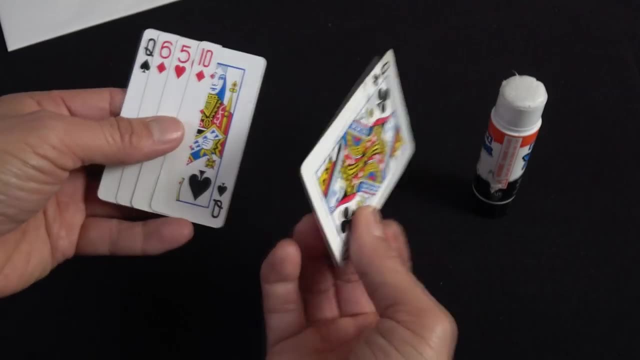 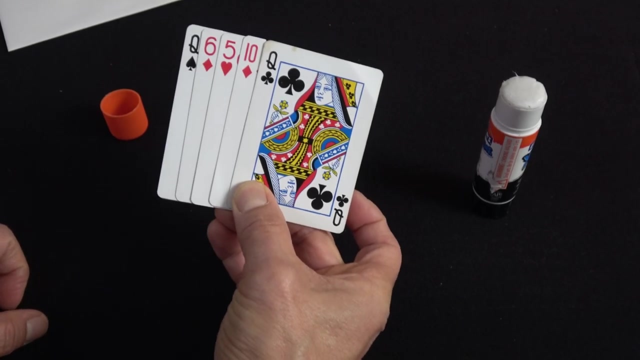 Once again, a Queen of Spades. back to back and you have three parts of a card there, And the secret to the whole thing is that when you hold another real card on top, it looks like you're displaying five cards. 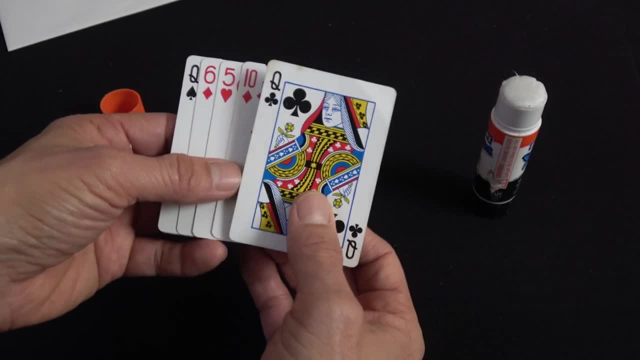 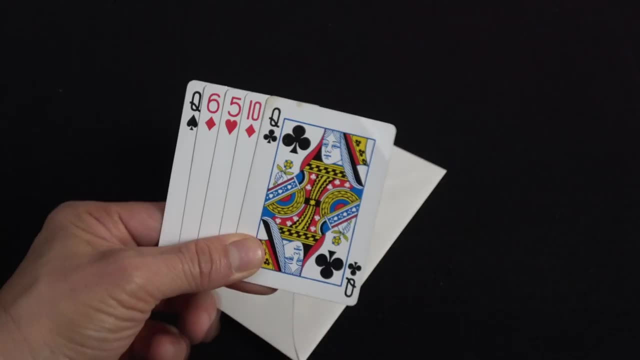 But you only have two. Now let's get to the explanation of the trick. Line up your cards and you're ready to perform the trick. Show your five cards. Just point out that you have the two queens there that are going to perform some magic. 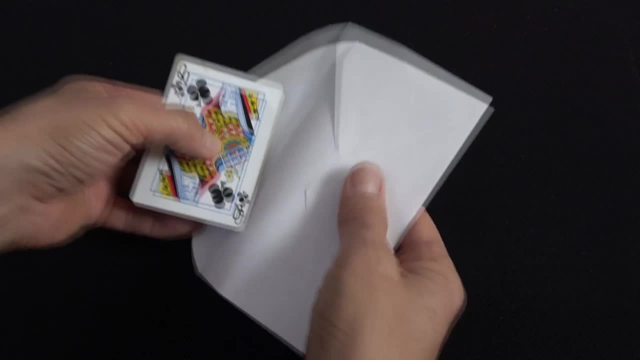 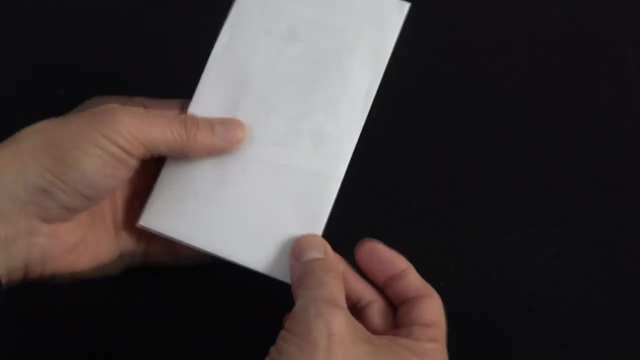 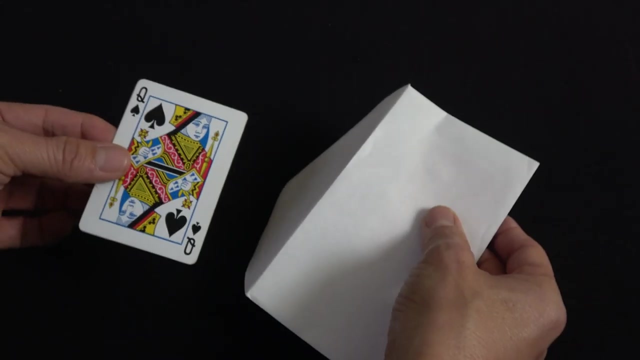 for the spectator. Fold the cards up, Place them inside of the envelope. the envelope, and now for the magic. turn the envelope over, snap your finger and then you're going to remove a couple cards. you're going to remove the queen. 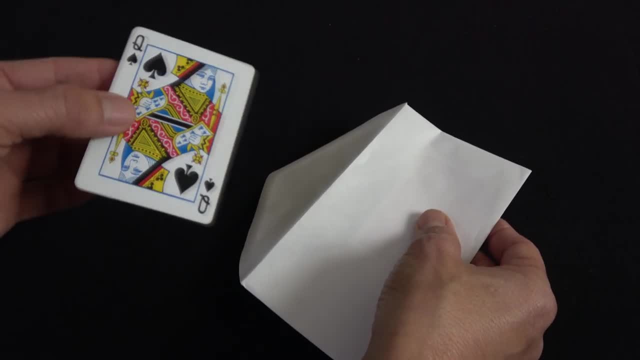 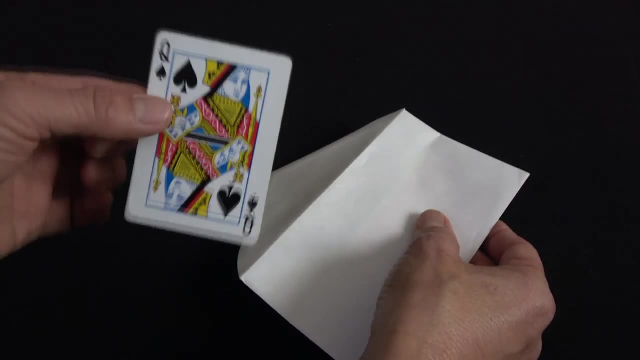 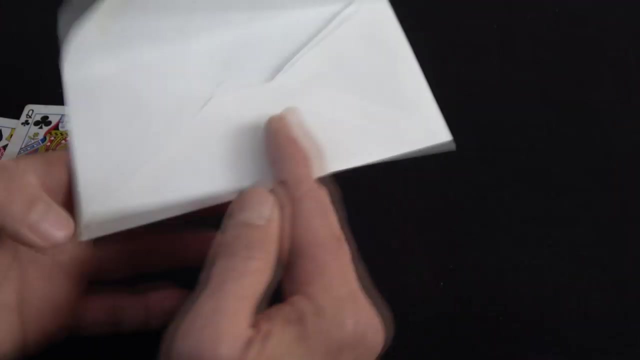 of spades. but what the spectators don't know is that when you turned over the envelope, you turned over the gimmick card and on the back is something that looks like this: that's the secret. so you take out the queen, take out the other Queen, and then you can show the envelope is empty. you can tear it up, have specter. 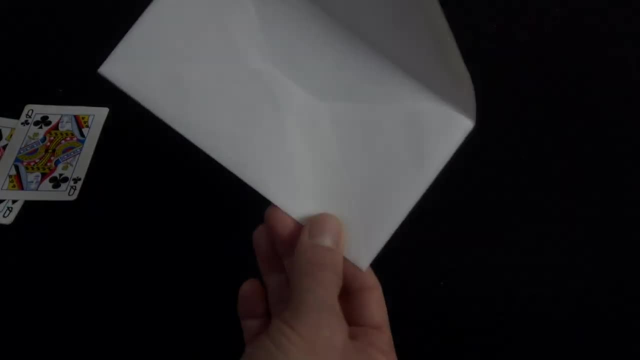 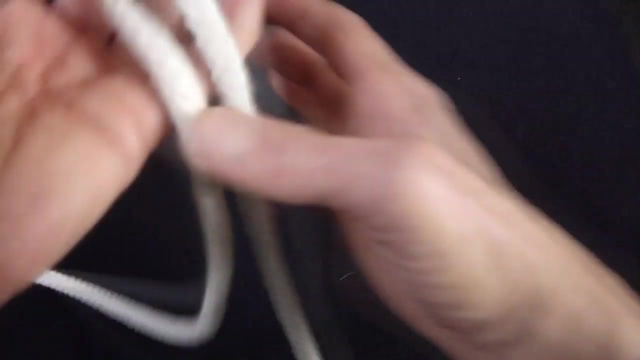 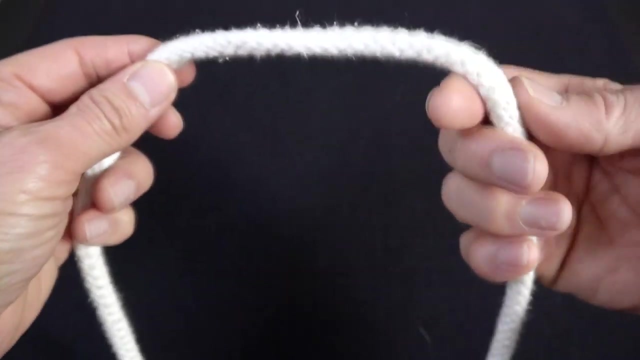 examine it and the cards- the three other cards- have vanished. here's a vanishing knot. you can do this with pretty much any length of rope. two to three feet is probably about right, though you don't want a 50 foot rope to do this now with. 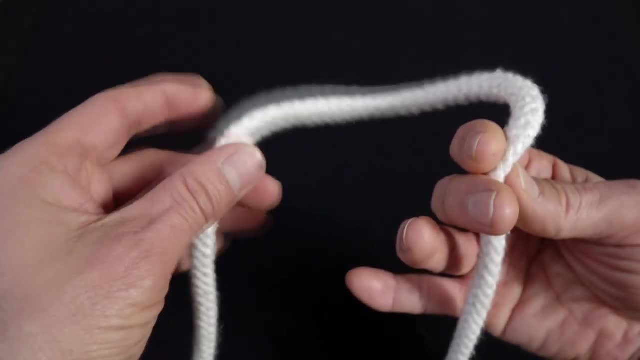 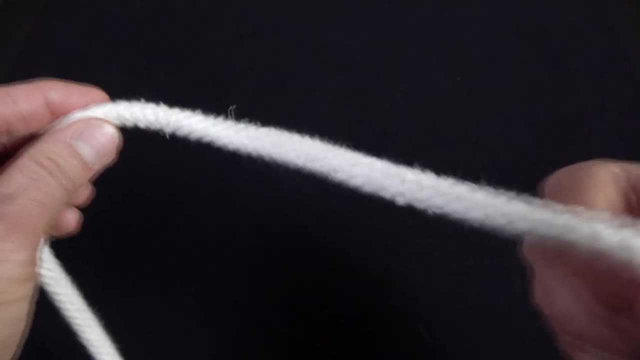 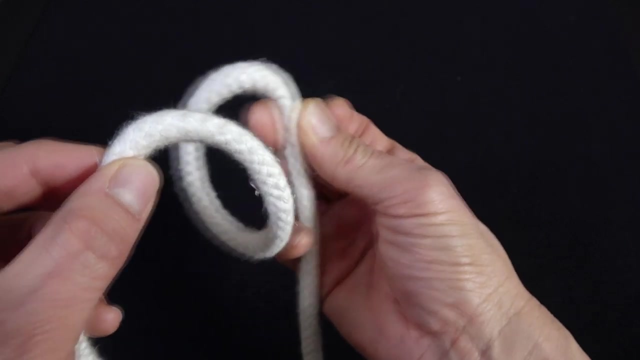 a greater reach. you can do it with pretty much any length of loop. so here's my hand right now. so I'm holding the rope this way with my fingers and thumb. left hand is just holding it between my first finger and thumb. now you're going to make a loop like this, so let's watch my right hand. it just kind of sweeps. 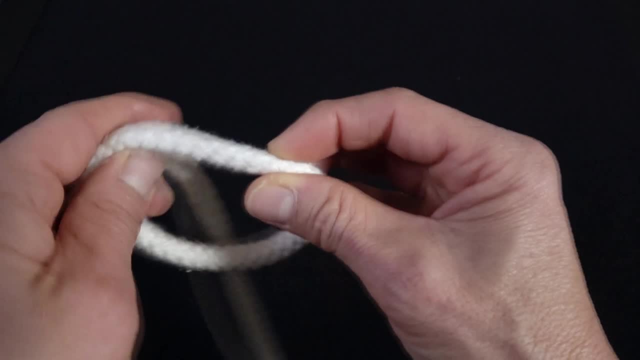 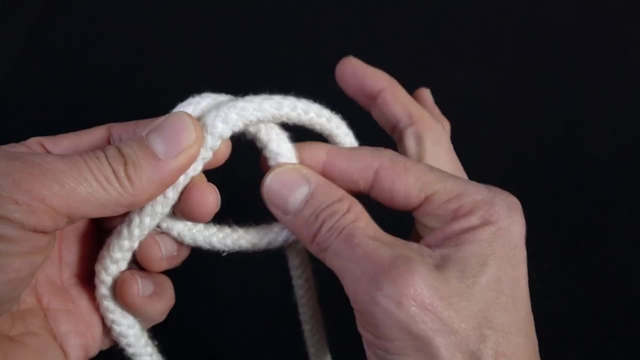 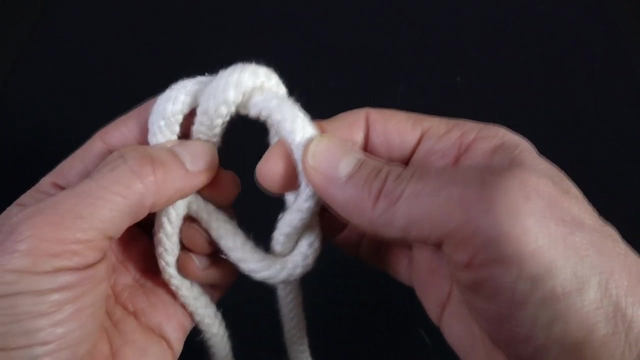 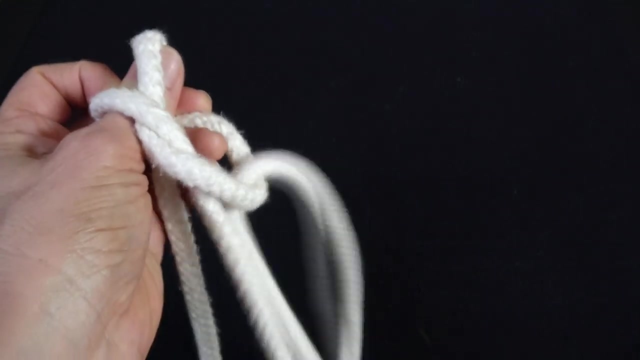 under and goes up. so the loop looks like this: hold the loop with your left hand here. now. here's the crucial part, as I'm pulling the rope through. watch my left thumb. it actually pushes this little bit of material through. so I push through. I run the rest of the rope. 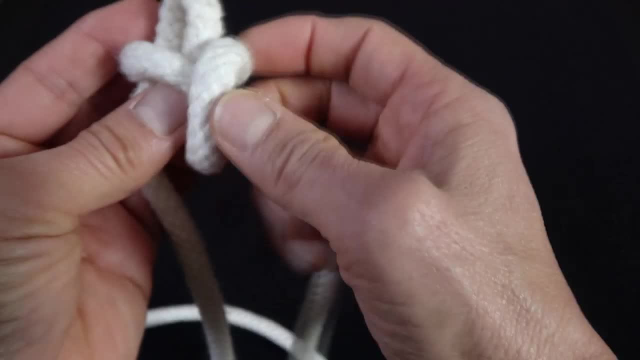 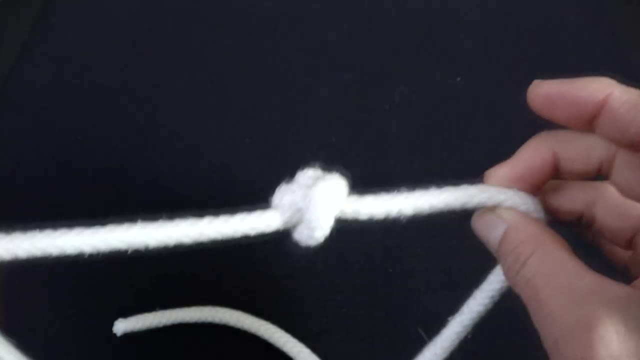 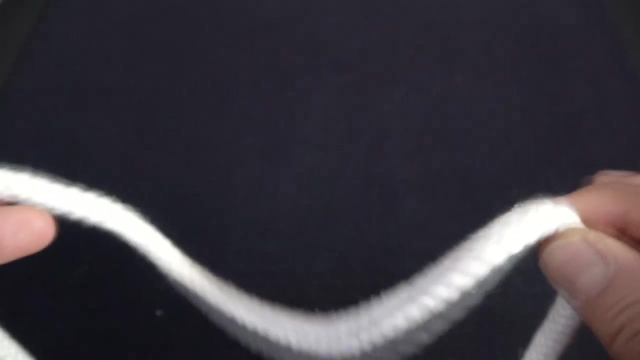 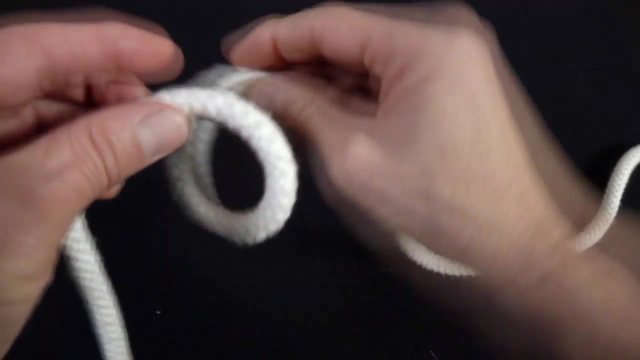 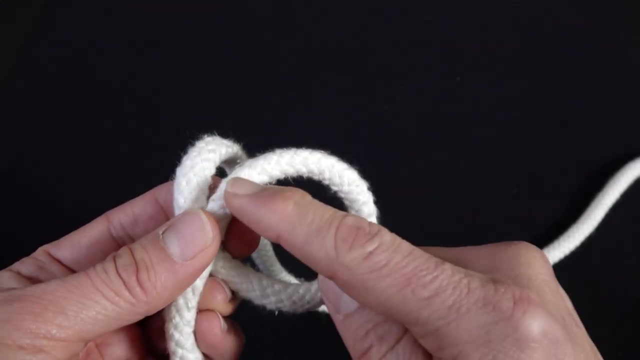 through and now I can tighten things up and it looks like a knot. however, you know there's a magic trick: if I pull, the knot vanishes. so once again, right hand, I kind of turn my hand towards me and sweep it under, creating a loop. now it's kind of important here to make sure that this part of the rope is to the right of this part. 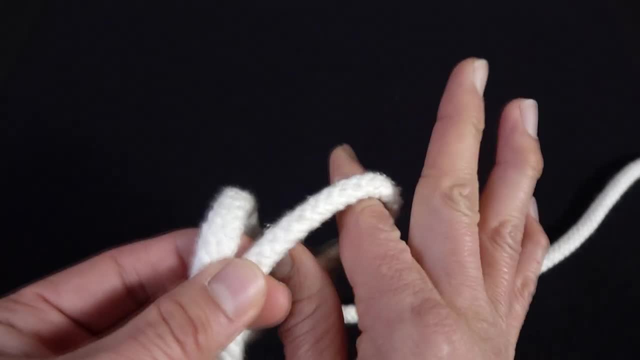 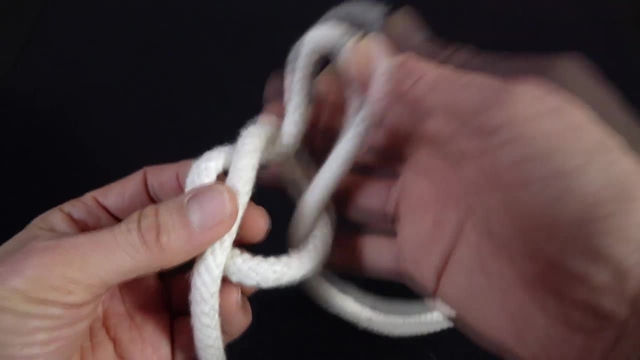 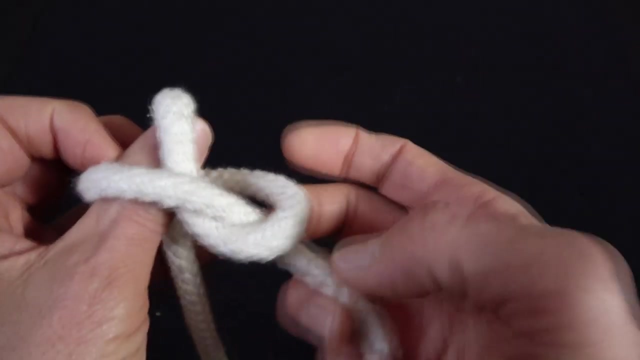 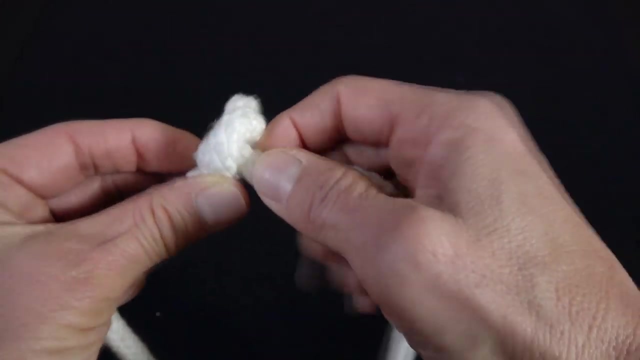 of the rope. rope, hold it, reach through with the finger and thumb, grab the end, pull it through and then the left thumb, right here, is pushing that through as I pull the rope through. now you pull on this end, this end, with my right hand. you pull that and you tighten everything up so it looks like a knot. 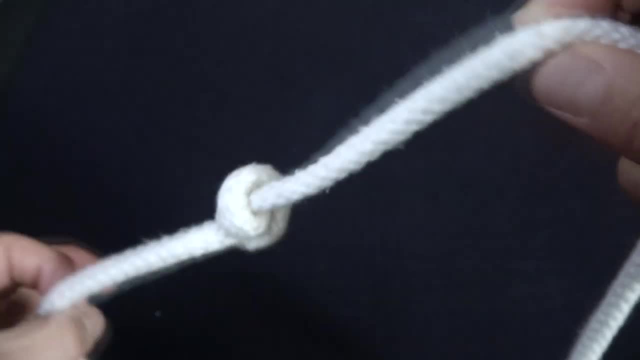 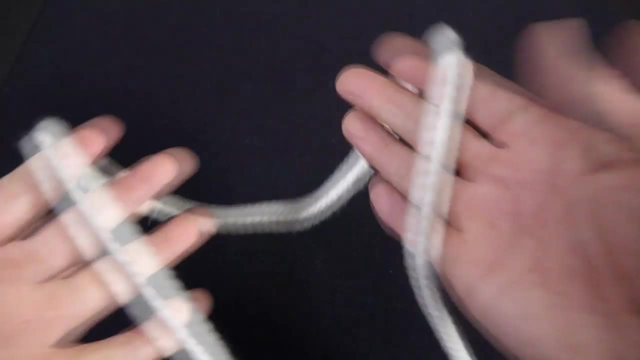 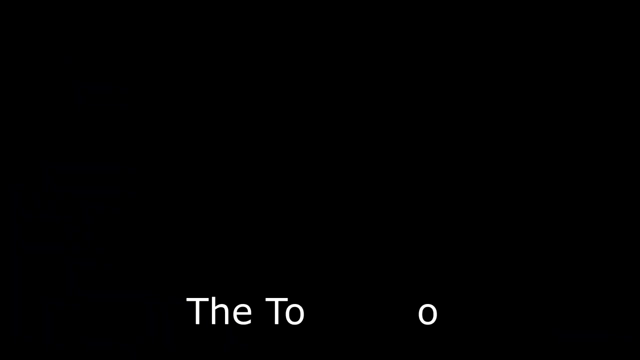 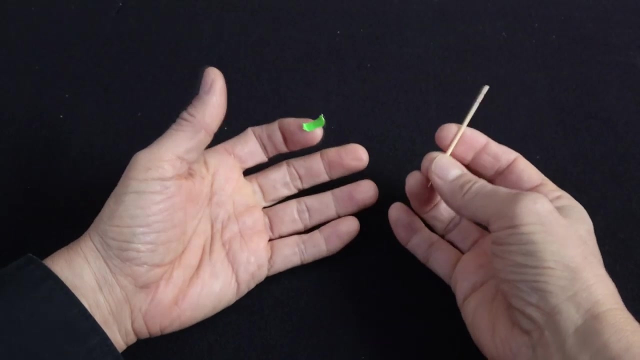 something in magic. you don't want this to come undone yet because you want spectators think you have a knot in your hand right here and then by pulling one, two, three, magic- the knot vanishes. what you'll need for this toothpick trick is a toothpick and a piece of tape. now I would suggest.